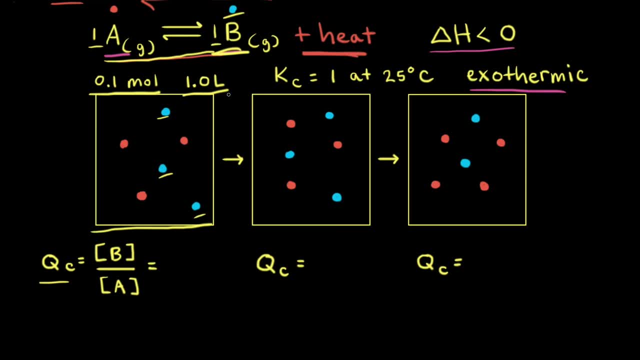 0.3 divided by 1.0 liter is 0.3 molar, So the concentration of B is equal to 0.3 molar. There are also three particles of A. therefore, the concentration of A is also equal to 0.3 molar. 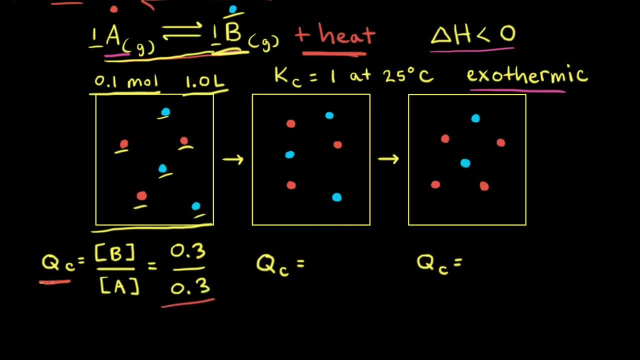 0.3 divided by 0.3 is equal to one. So QC at this moment of time is equal to one. KC for this reaction is equal to one at 25 degrees Celsius. So QC is equal to KC. And when QC is equal to KC, 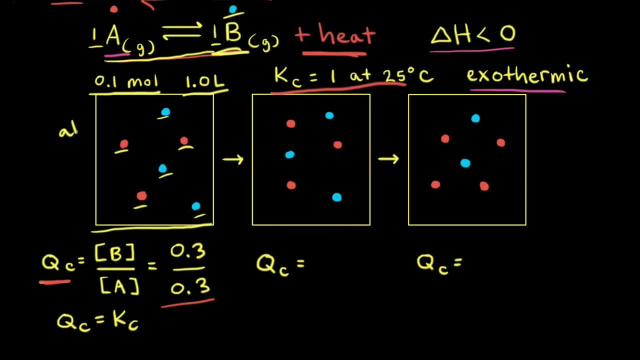 the reaction is at equilibrium. So for this first particulate diagram the reaction's at equilibrium. Next we introduce a stress to the reaction at equilibrium and the stress is an increase in the temperature In general for an exothermic reaction. 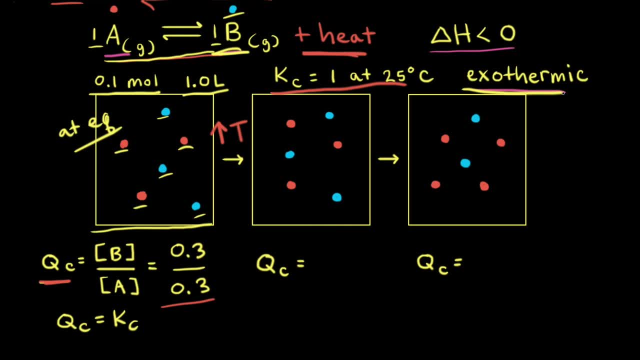 increasing the temperature lowers the value for the equilibrium constant. So for this hypothetical reaction, at 25 degrees Celsius KC is equal to one, But since we've increased the temperature, the value for the equilibrium constant is going to decrease. So let's say it goes to 0.5. 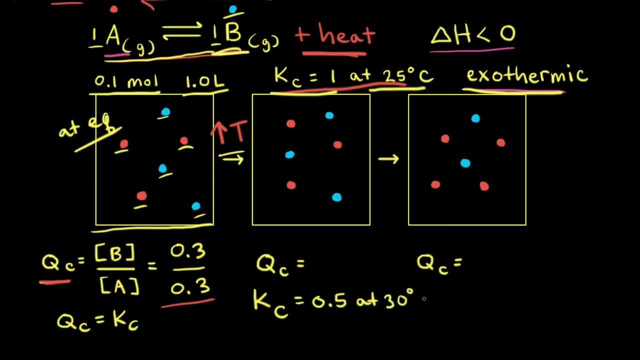 if we increase the temperature to 30 degrees Celsius. So if we calculate QC for our second particulate diagram, we still have three blues and three reds and the volume is still the same. Therefore, QC is still equal to one, But the difference is KC has now changed. 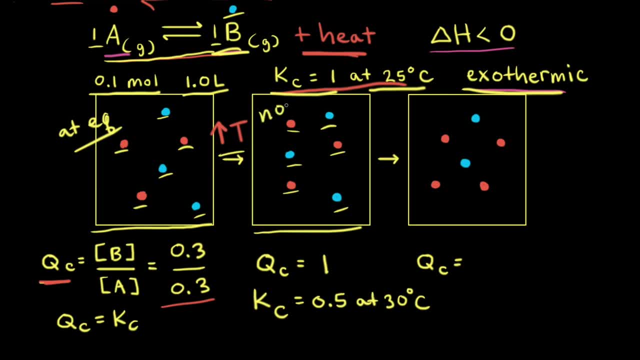 So QC is not equal to KC, So QC is not equal to KC, So we are not at equilibrium. And in this case QC is greater than KC because QC is equal to one and KC is equal to 0.5.. And when QC is greater than KC, 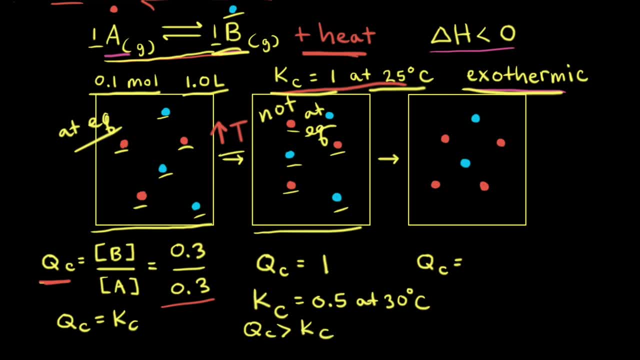 there are too many products and not enough reactants And therefore the net reaction goes to the left. When the net reaction goes to the left, we're going to have B turn into A. So we should see one blue sphere turn into one red sphere. 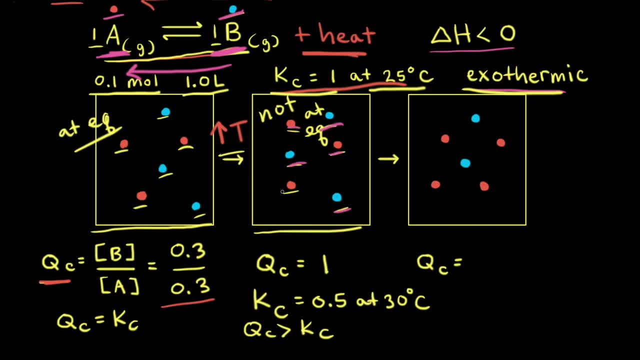 So if we have three blues and three reds and one blue turns into a red, that gives us only two blues and four reds now. So when we calculate QC for our third particulate diagram, the concentration of B would be 0.2 molar. 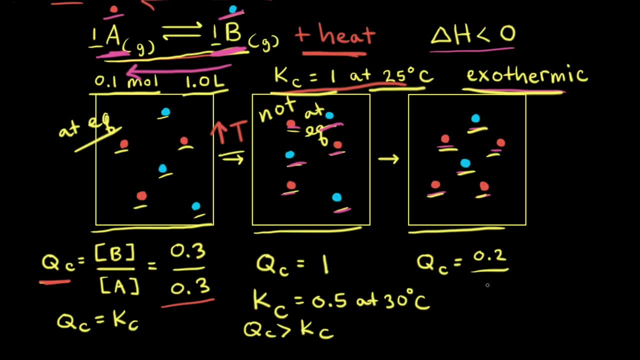 and the concentration of A would be 0.4 molar. So 0.2 divided by 0.4 is equal to 0.5.. Well, KC is also equal to 0.5.. Therefore, QC is equal to KC. 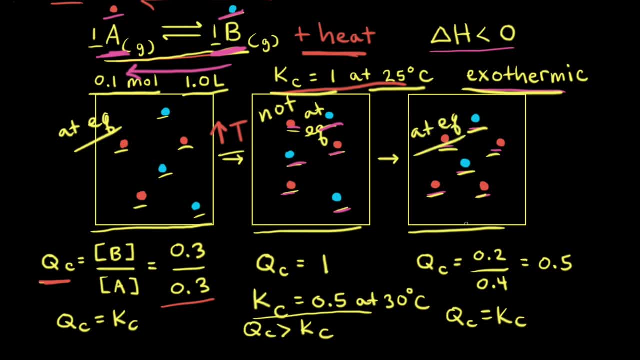 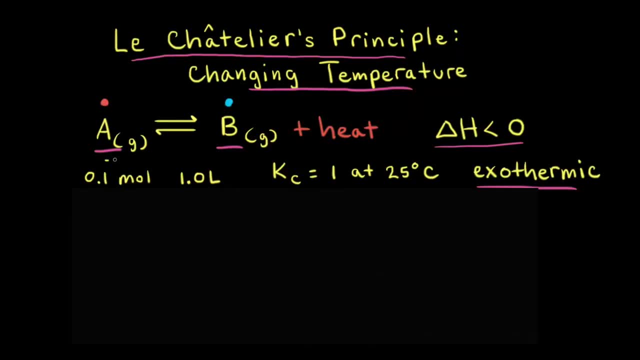 and the reaction is at equilibrium, And when a reaction is at equilibrium, the concentrations of reactants and products are constant. Let's go back to our hypothetical reaction at equilibrium, but this time we're going to decrease the temperature If we treat heat like a product. 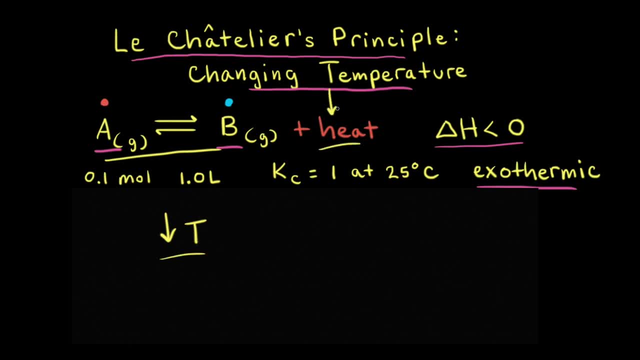 decreasing the temperature is like decreasing the amount of one of the products. Therefore, the net reaction will go to the right to make more product. If we approach this problem by thinking about the reaction quotient Q for an exothermic reaction, a decrease in temperature in general causes an increase. 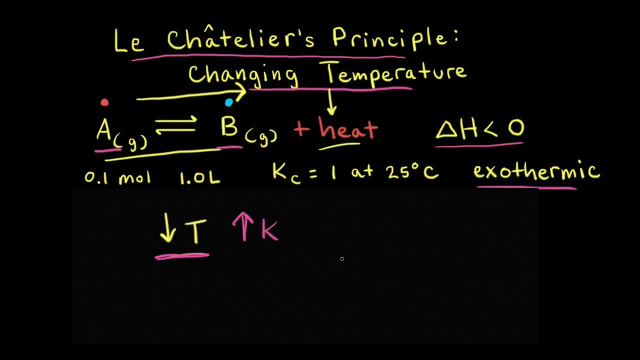 in the equilibrium constant And if the equilibrium constant increases, then Q would be less than K, And when Q is less than K, the net reaction goes to the right. The net reaction would continue to go to the right until Q is equal to K. 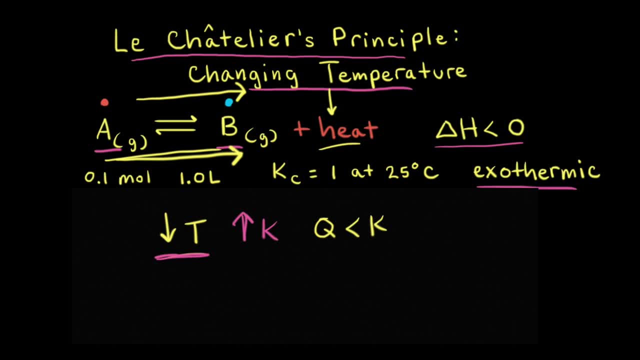 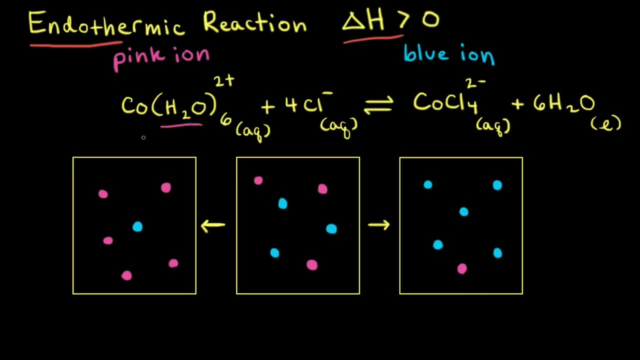 And equilibrium has been reestablished. Next, let's look at an endothermic reaction where delta H is greater than zero, When six water molecules complex to a cobalt two plus ion, the resulting complex ion is pink in color. And when four chloride anions complex, 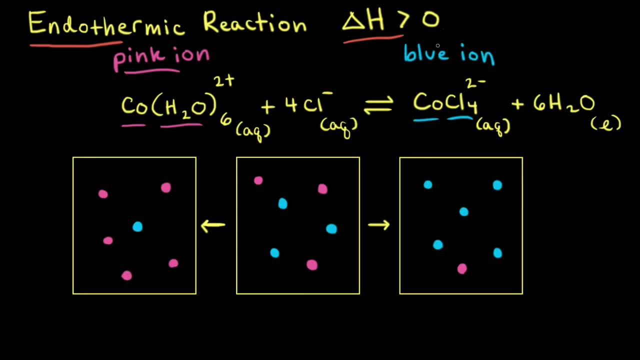 to a cobalt two plus ion, the resulting complex ion is blue in color. When the pink ion reacts with four chloride anions, the blue ion is formed, And since this reaction is endothermic, we can put heat on the reactant side. 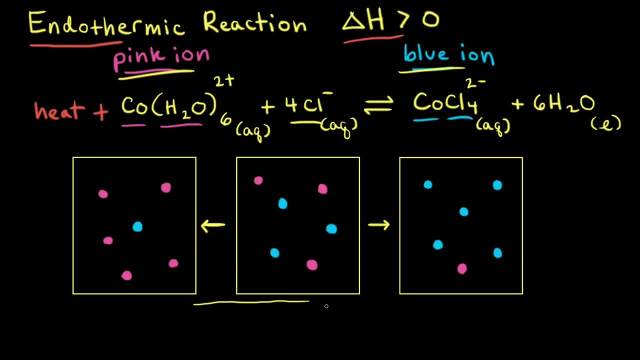 We're gonna use these particular diagrams down here to help us understand what happens to an endothermic reaction at equilibrium when the temperature changes. However, these drawings aren't designed to be completely accurate for this particular reaction. They're just to help us understand what color we would see. 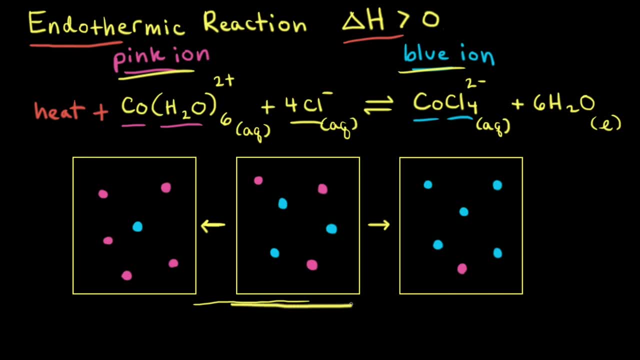 For example, let's say that this middle particulate diagram represents the reaction at equilibrium, And if there are decent amounts of both the blue ion and the pink ion at equilibrium, the resulting equilibrium mixture- so this is an aqueous solution- would appear to be purple or violet. 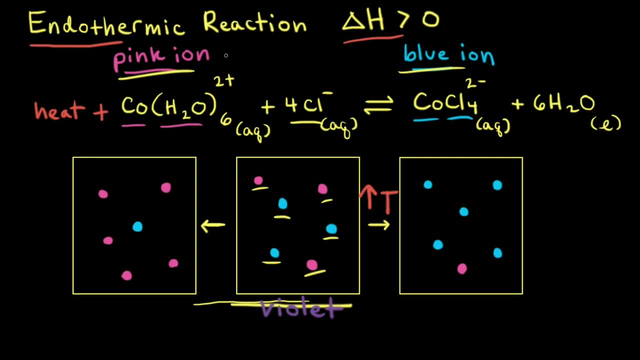 If we were to increase the temperature for this endothermic reaction? we treat heat like a reactant, So increasing the temperature is like increasing the amount of a reactant And therefore the net reaction will shift to the right to get rid of some of that reactant. 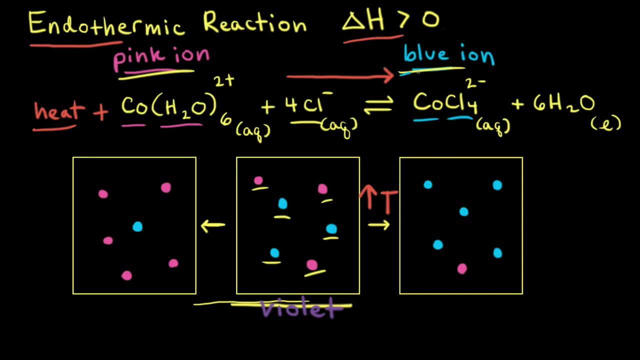 When the net reaction goes to the right, we're gonna increase in the amount of blue ion and we're going to decrease in the amount of pink ion. Therefore, looking at this particulate diagram on the right, there are now more blue ions than there are pink ions. 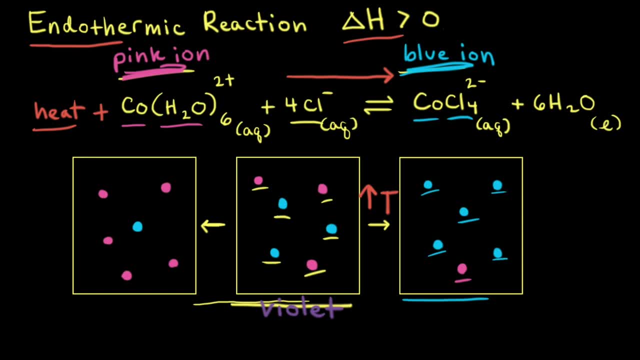 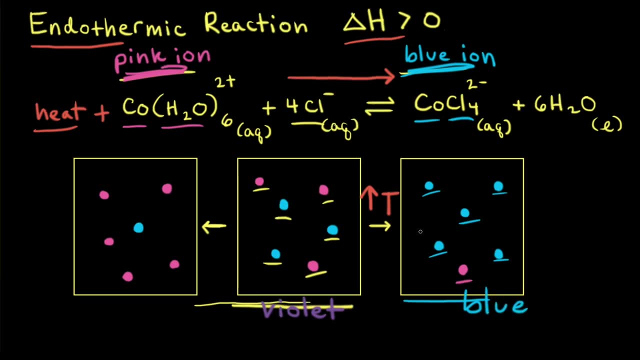 compared to our equilibrium mixture in the middle. Therefore, for this third particulate diagram, the resulting aqueous solution is going to look blue. If we think about this, using Q in general for an equilibrium mixture, we're gonna have blue In general for an endothermic reaction. 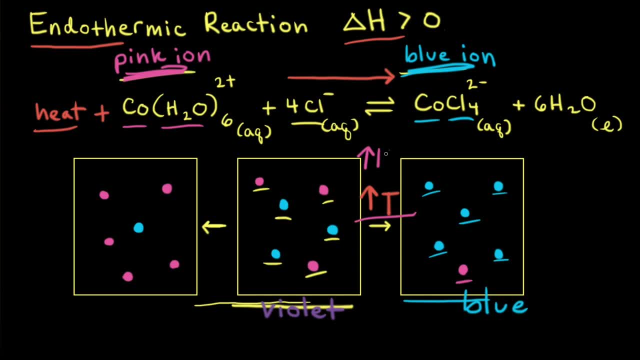 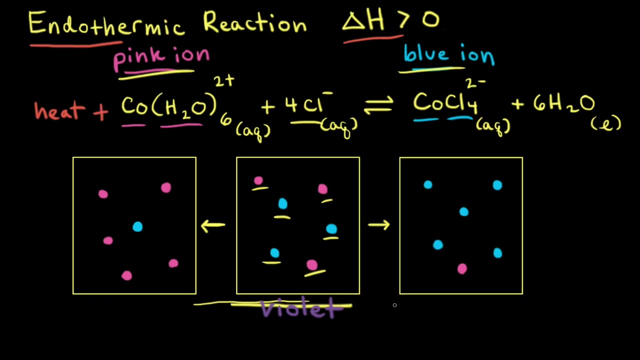 an increase in temperature causes an increase in the equilibrium constant K, And if K increases, then the reaction quotient Q is less than K, And when Q is less than K, the net reaction goes to the right. Now let's go back to the middle particulate diagram. 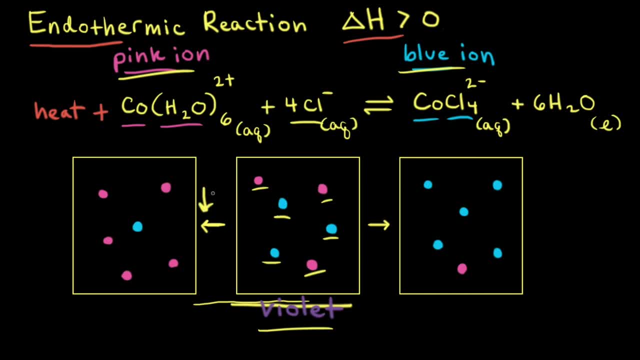 And so there are reactions at equilibrium, and this time we're going to decrease the temperature. If we treat heat as a reactant and we decrease the temperature, it's like we're decreasing one of our reactants. Therefore, the net reaction will shift to the left. 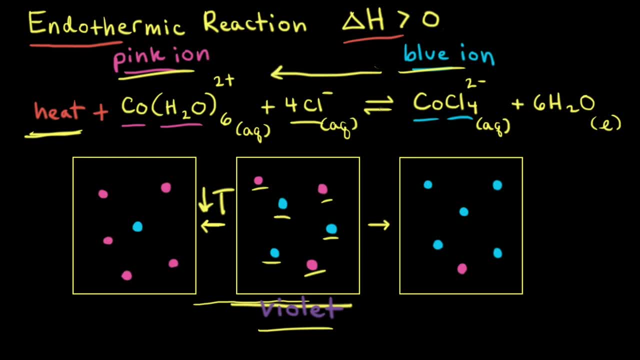 to make more of our reactant. And when the net reaction goes to the left, we're gonna decrease in the amount of the blue ion and we're going to increase in the amount of the pink ion. So when we compare the middle particulate diagram, 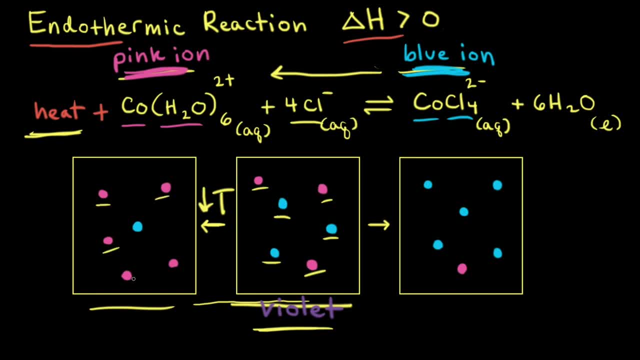 to the one on the left and the one on the left, there's a lot more of the pink ion than there is of the blue ion. Therefore, the overall solution, the overall aqueous solution, is going to be less than K. 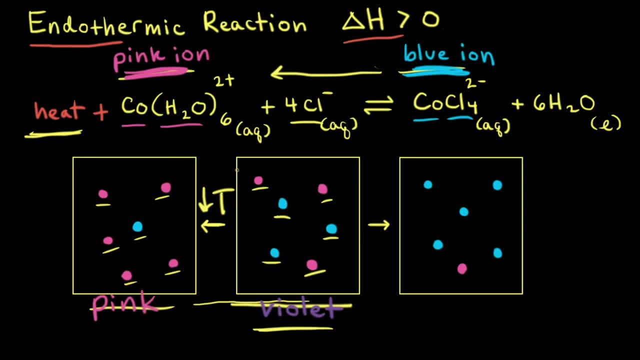 The aqueous solution is going to appear pink. If we think about what's happening using Q for an endothermic reaction in general, when you decrease the temperature, you decrease the equilibrium constant, And if the equilibrium constant decreases now, Q would be greater than K. 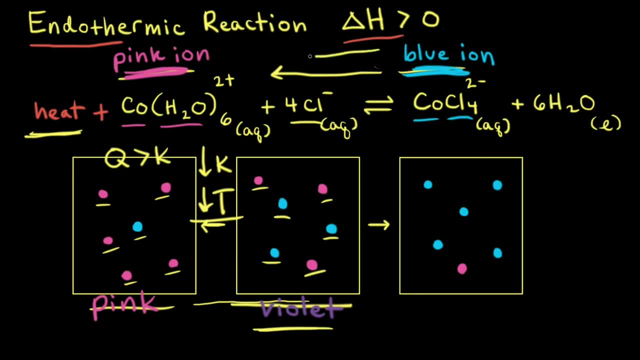 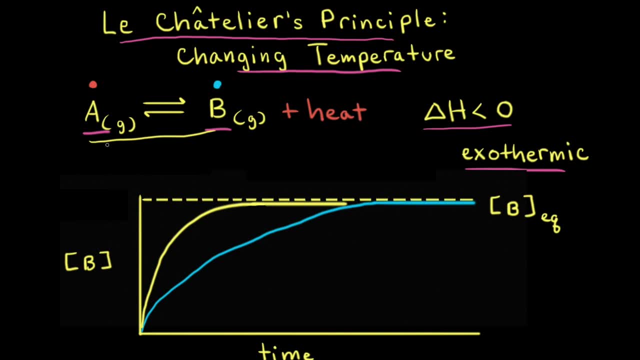 which means too many products and not enough reactants. Therefore, the net reaction would go to the left. Let's go back to our exothermic reaction At this time. let's pretend like we're starting with only A. So we start with only A and we have none of B. 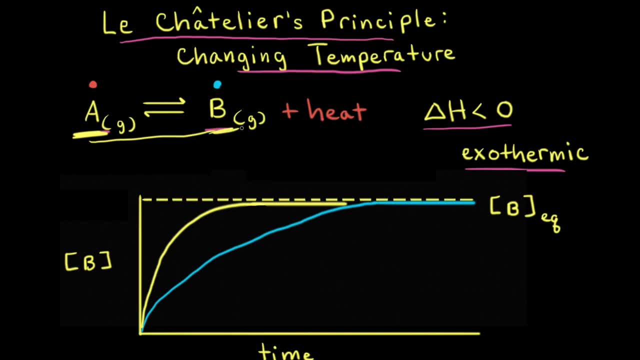 And our goal is to make as much B as we possibly can and to do it as fast as possible. One way to increase the rate of a reaction would be to increase the temperature. However, for an exothermic reaction, increasing the temperature decreases the equilibrium constant K. 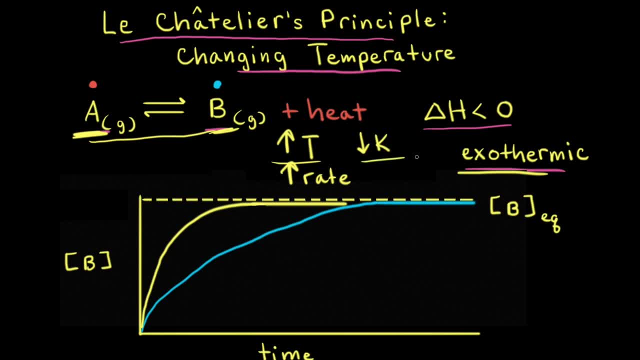 And if you decrease the equilibrium constant K, you would decrease the amount of B that you would have when you reach equilibrium. So we can't run our hypothetical reaction at too high of a temperature because that would decrease the equilibrium constant. So instead to speed up the rate of the reaction, 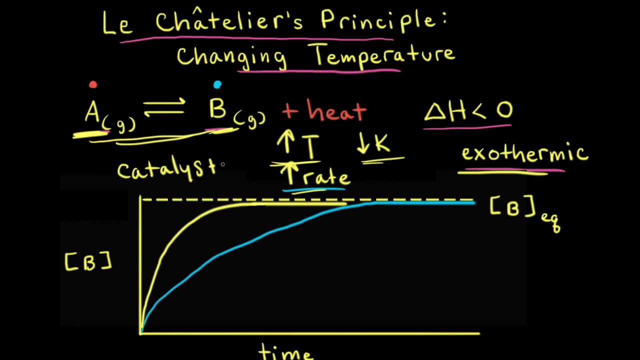 we could add a catalyst. Let's look at a graph of concentration of B versus time And we're gonna start with this blue curve here, which represents the hypothetical reaction without a catalyst, so the uncatalyzed reaction. When time is equal to zero, the concentration of B is zero. 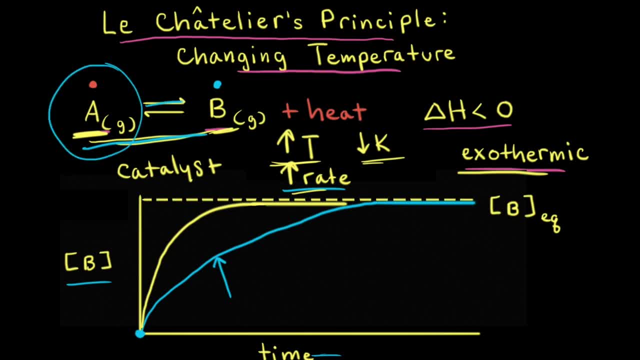 because we start with only A. So when A turns into B, the concentration of B increases over time and eventually the concentration of B becomes constant. And when the concentration of B becomes constant, the reaction reaches equilibrium. So this dotted line here represents: 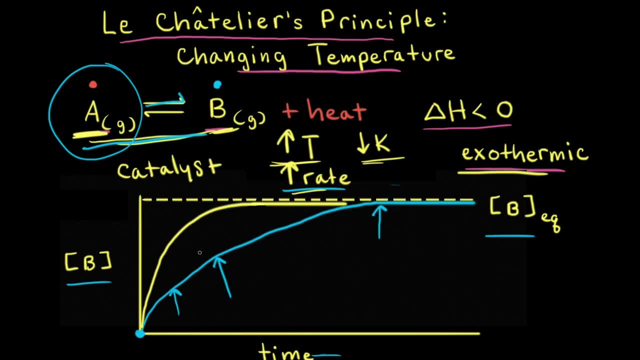 the concentration of B at equilibrium. The yellow line represents the reaction with a catalyst added. So once again we're starting with only A. So when time is equal to zero, the concentration of B is equal to zero, And as time increases, A turns into B. 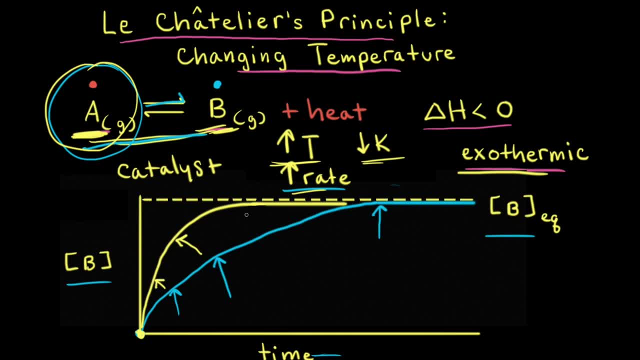 So the concentration of B increases And eventually the concentration of B becomes constant and the reaction reaches equilibrium. Notice that the reaction reached equilibrium much faster with the addition of the catalyst than it did without the catalyst. So the addition of a catalyst allows a reaction. 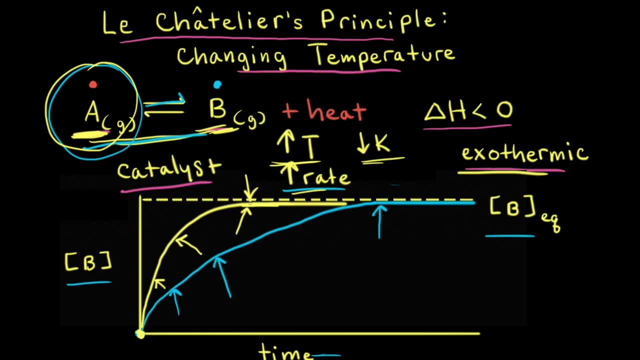 to reach equilibrium faster. However, notice that the final equilibrium concentration of B is the same for both the uncatalyzed reaction and the catalyzed reaction. Therefore, the addition of a catalyst does not change the composition of the equilibrium mixture, And that's because the catalyst speeds up. 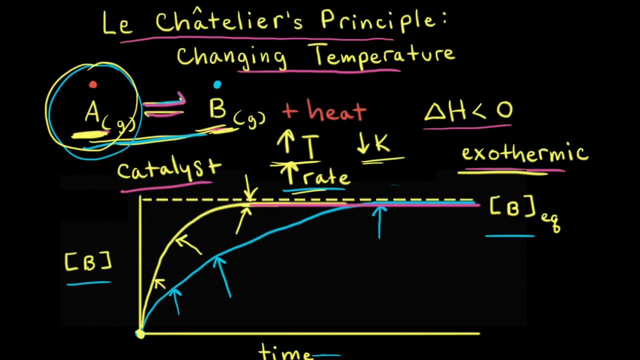 both the forward reaction and the reverse reaction, but the rates are still equal. And since the rates are equal, there's no change in the composition of the equilibrium mixture.